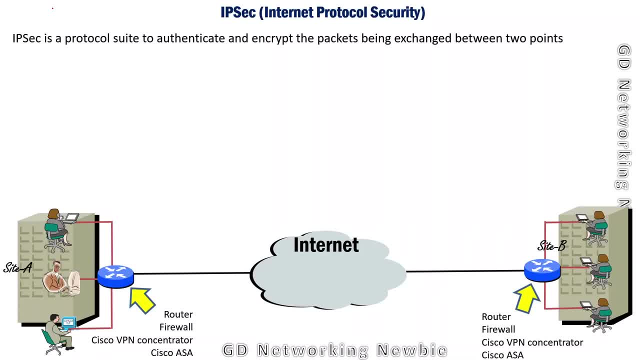 Hi everyone. in this video we are going to discuss about IPSec, and IPSec it stands for Internet Protocol Security. Now, this IPSec is a protocol suite that is used to authenticate and encrypt the packets which are being exchanged between two points, For example, in our case. 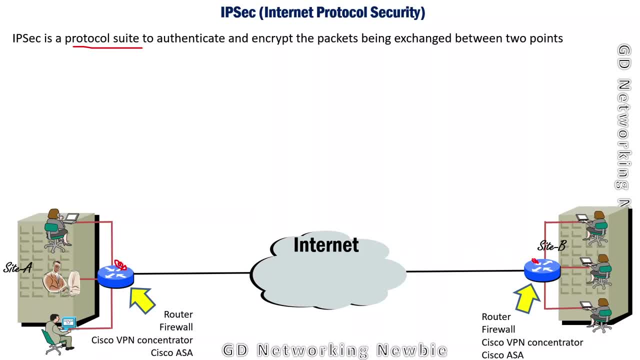 let's say this is router 1,- one point- and this router 2, this is the second point. Now, if you want to send some data in between these two points securely, then we can use IPSec, And we also discussed in our previous video that VPN, which stands for virtual private. 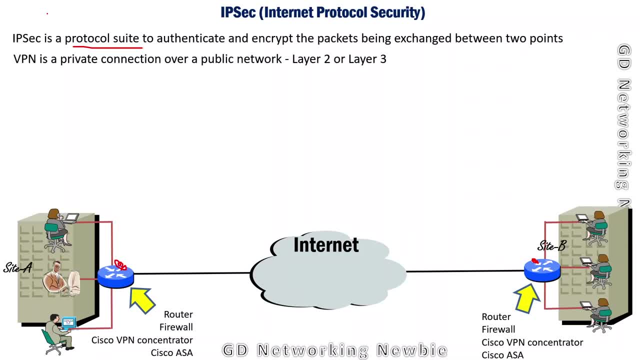 network is actually a private connection over the public network. So what happens here is this private connection will be established using public network, like the internet, and that private network will provide us with a uma, upgrades or entity Salem Now stumble to send our information securely from one point to another. Now this tunnel or 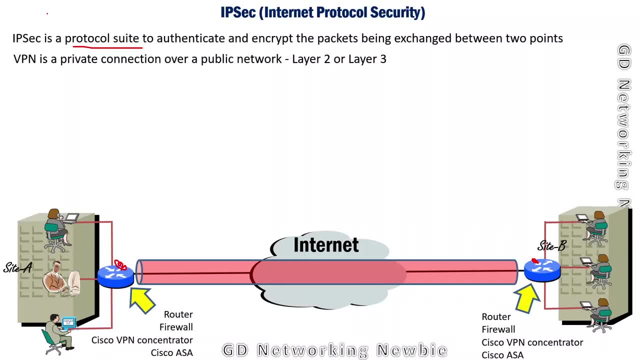 this virtual connection can be created using layer 1 or at layer 1, sorry, layer 2 or layer 3, and when we create this virtual tunnel at layer 3, we use IPSec. Now IPSec actually provides us integrity for our message. so 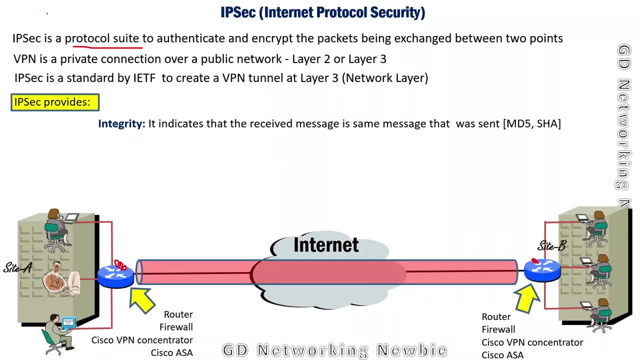 integrity indicates that the received message is actually the same message which was sent from the transmitting end. It means the contents of the message has not been changed, and to achieve this integrity we can use this algorithm, like MD5 or SHA, And IPSec also provides us authentication, and authentication refers to verifying the 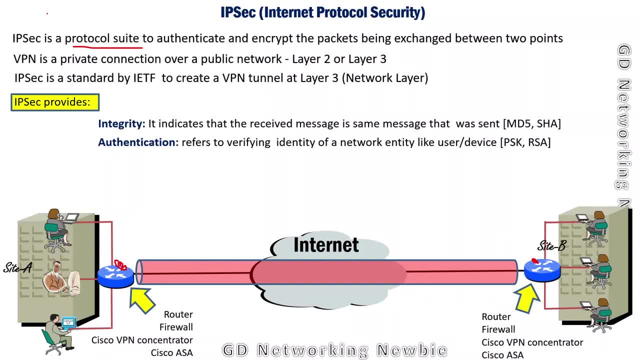 identity of the message, The identity of the network entities like user or devices. so we want to authenticate that the sender is really the one from where we were expecting. so, like the answer to question that who you are, They prove the identity and for that we can use maybe PSK pre-shared key or RSA algorithm to authenticate the. 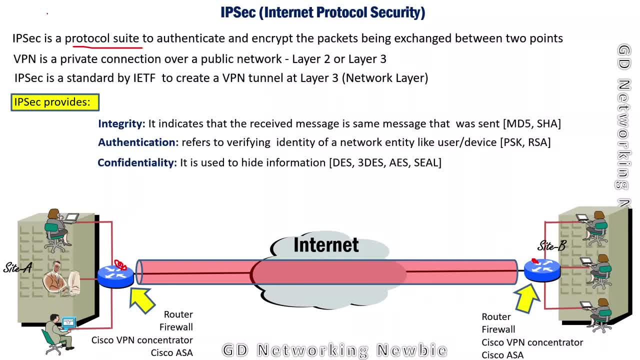 users. IPSec also provides confidentiality and confidentially actually refers to the message that was sent to the sender. And IPSec also provides confidentiality and confidentially actually refers to the message that was sent to the sender. And IPSec also provides efforts to hiding the information. so we want to send our information hidden, so 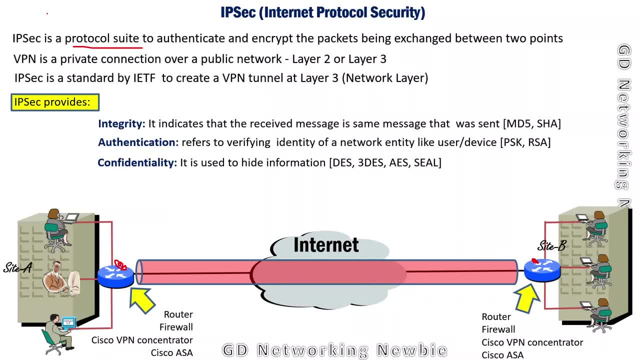 that no unauthorized user can access to our information or can read our information, And for confidentiality we use different encryption algorithm like DES, triple, DES, AES or SEAL, And this IPSec also provides key management. so for the secure communication, for encryption or for different things, we 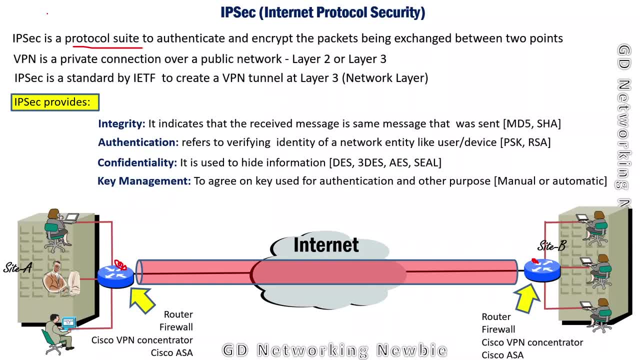 need keys and both the transmitting and the receiving end, And that key management is done by some specific protocol we will discuss on the next slide. So key management is to agree on a key used for authentication and for other purpose, and that could be done by manual or that could be automatic. So these are. 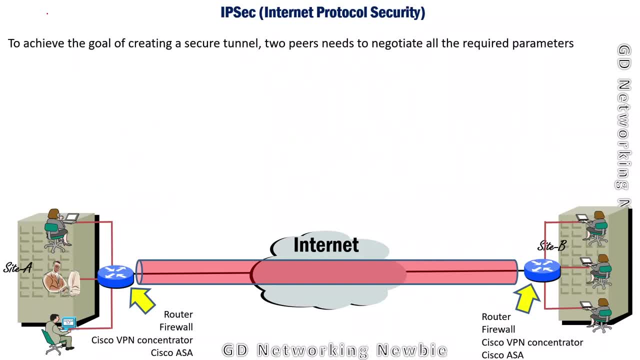 the different things provided by IPSec. And now let's say that now, to achieve the goal of creating a secure tunnel, these two pairs, for example, in our case, router 1 and router 2- they need to negotiate all the required parameters to provide us the confidentiality, integrity, authentication and secure key exchange. 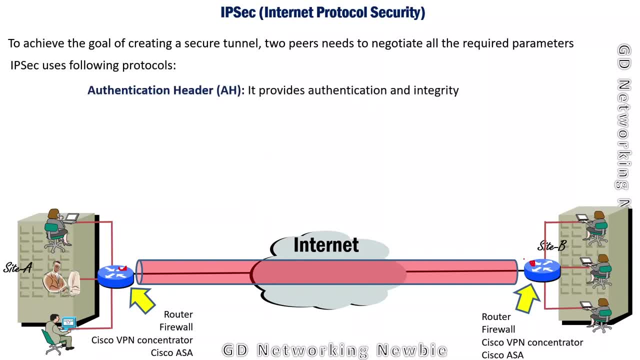 so for that, this IPSec uses the following protocol to achieve these all things. it uses authentication header, and this authentication header is actually an encapsulation- we'll discuss in detail in our next video- but it actually provides authentication and integrity for our messages being sent between these two points. and then it also it can also use encapsulation. 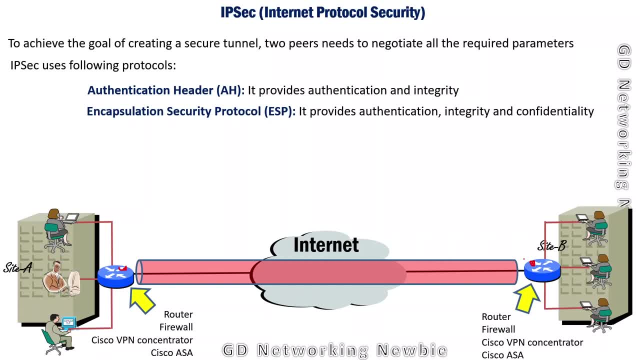 security protocol, ESP, and so ESP provides authentication, integrity and additional security for our messages. The additional thing is the confidentiality, which is provided by ESP, but AHR authentication header does not provide this one, so confidentiality is the additional thing, Authentication, integrity are same, and confidentially. 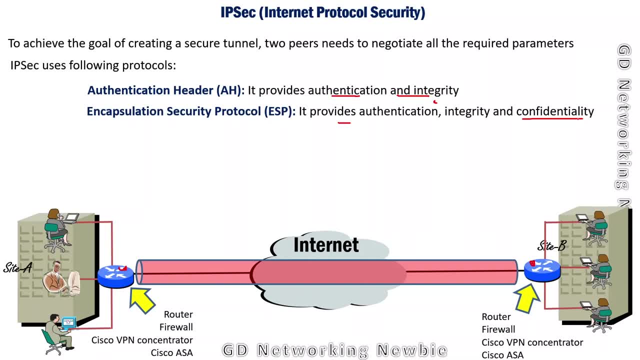 confidentiality is provided by encapsulation security protocol. so both of them are encapsulation protocol. so at one time we will be using maybe AH or ESP so and maybe something like that. Maybe sometimes we can combine them as well. so these are two encapsulation protocols which are defined in this IPSec framework. Now, and the third thing is: 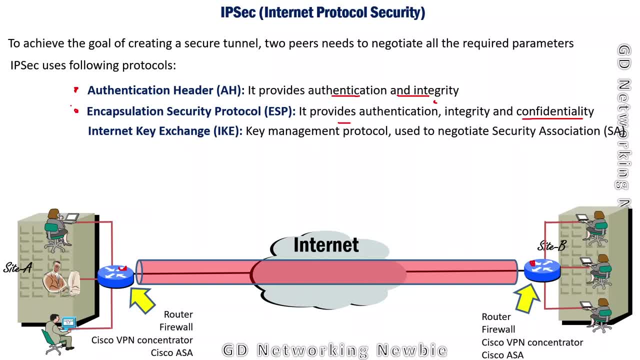 Internet key exchange. so Internet key exchange is a key management protocol and that protocol is used to negotiate the security association, security association between these two points. these, for example, in this case these two routers. they want to communicate with each other. These are our peers and they will exchange the security association using iInternet Key. 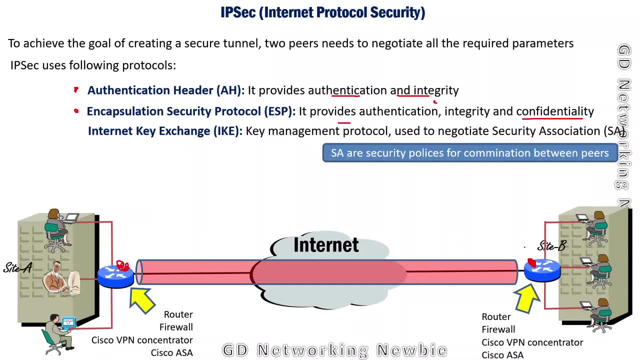 Exchange Protocol. Now, security associations are basically security policies for communication between peers, So this will be communication. I have made a mistake maybe in spelling. this is for communication between peers. Security policy for communication between these two routers is known as security association. 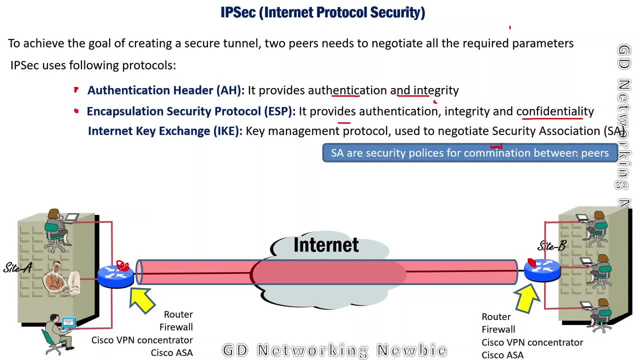 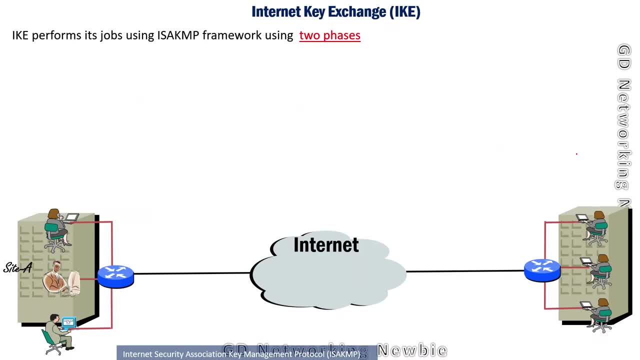 So this security association will be negotiated using IEC. Now IEC itself performs its job using IC-CAMP framework, and in that it uses two phases, and IC-CAMP actually stands for Internet Security Association Key Management Protocol, which I have written here Down. you can see here: 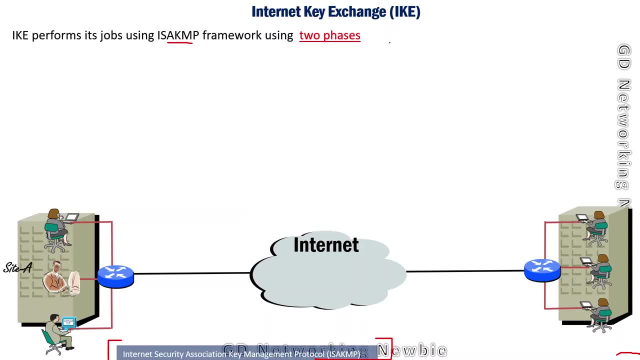 So IEC itself uses IC-CAMP framework and to negotiate the security association IEC uses two phases. IEC comprises of two phases and in the first phase this IEC uses this first phase to negotiate IC-CAMP policy, and for IC-CAMP policy it exchanges five parameters. 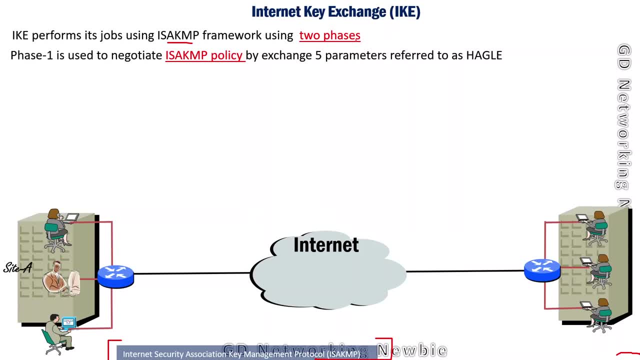 and they are referred to as Hegel, So H-A-G-L-E. so specifically, Hegel means they will be exchanging five parameters. like we can see, H is the hash value, so they will agree on a common hash value between these two points. 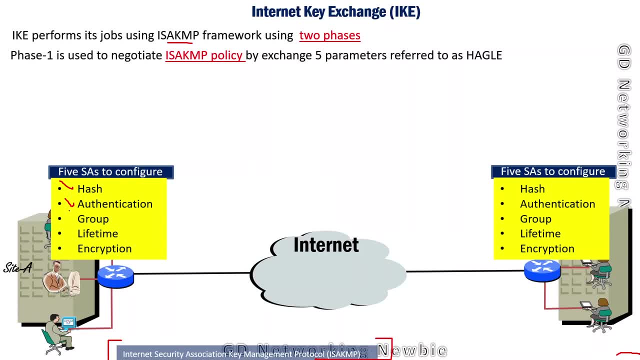 and then authentication, authentication mechanism- they also need to agree on a common authentication method- and then group Diffie-Hellman, group 4. And then also the lifetime of the IC, And then also the connection that how much time this channel will be active, or the connection. 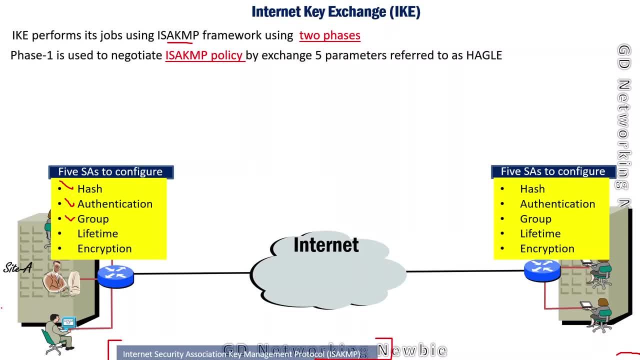 will be active and then also they decide about the encryption. So they need to have these common things in between these two nodes for creating a secure tunnel. So after this phase, pairs authenticate each other and they calculate a shared secret key by exchanging of these five parameters known as Hegel. 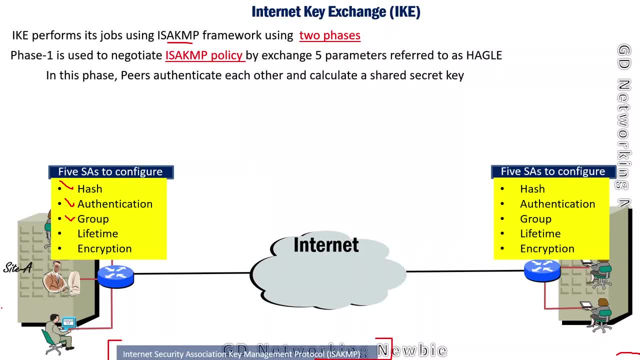 Okay, Now actually they are referred to as Hegel H-A-G-L-E And then by this exchange actually pairs negotiate, security associations, And after this negotiation actually they actually define or they agree on a common policy set. We call it IEC policy set or Internet Key Exchange Policy Set. 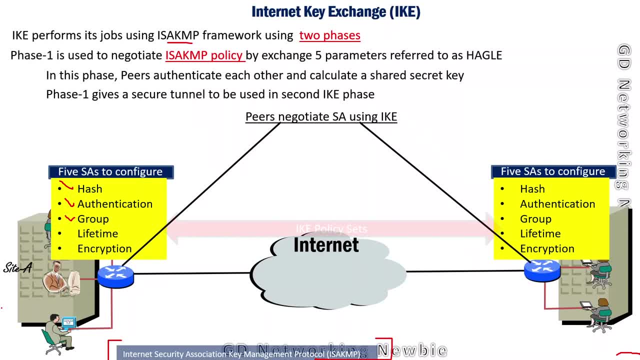 Now this phase, actually after this, gives a tunnel. So phase one gives a secure tunnel. That tunnel will be used for the second IEC phase, So they will have a tunnel like this one. And now, once we have this tunnel, we can move to the next phase or the second phase of IEC. 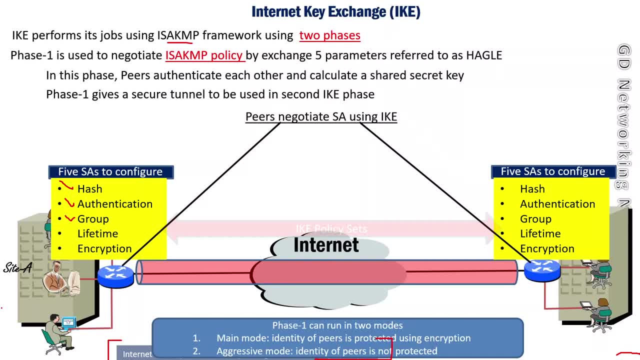 And yes, one point worth to mention here is that that this phase one can be configured to run in two modes. One mode is known as man mode and second mode is known as aggressive mode. The difference is that in the man mode, the identity of these pairs is protected by using 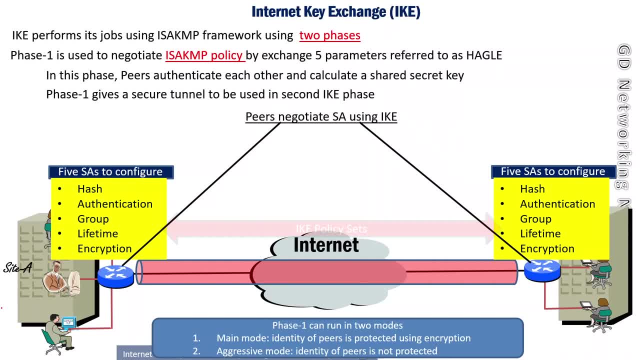 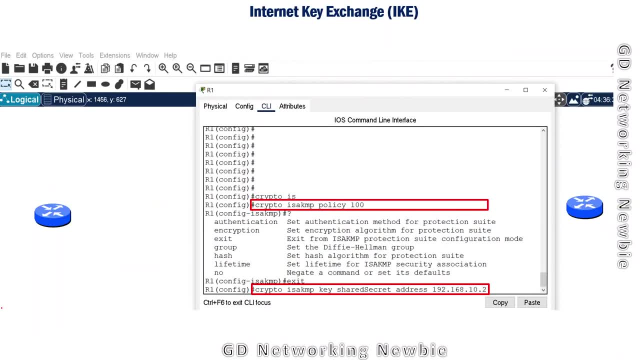 some encryption, But in aggressive mode the identity of pair is not guaranteed to be protected. So in these two modes, the phase one is run Now. if you see this, we will do this exercise in the packet tracer as well. Okay, 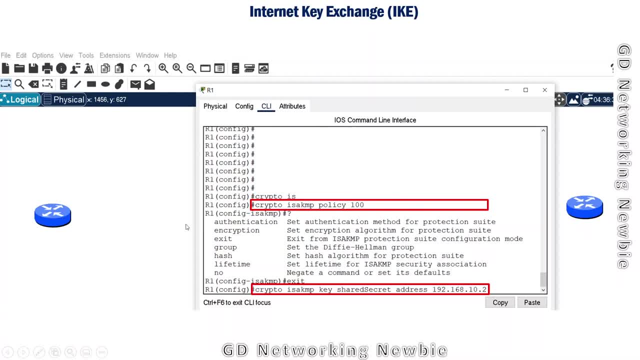 So let's say what they are exchanged in the first phase. just, I have given, I have shown you a simple snapshot here. So for this, for IEC and policy, we give some priority value here And then you can see these all five values which I mentioned there- H, A, G, L, E- they. 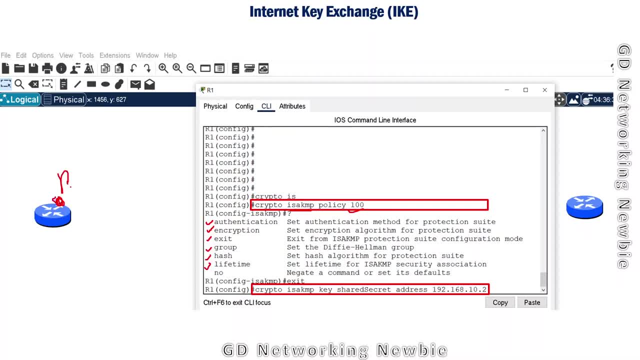 are configured both at this router, maybe R1. And this also needs to be configured at router two as well. So by using this common parameter, we can configure this as well. Okay, So let's see, Okay, Okay, Okay. 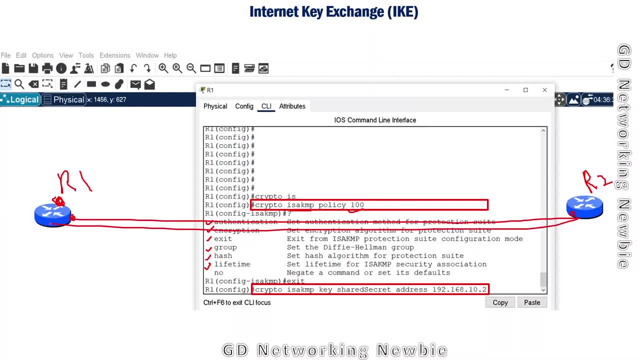 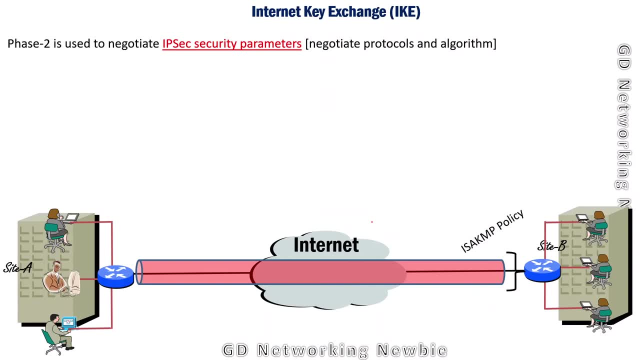 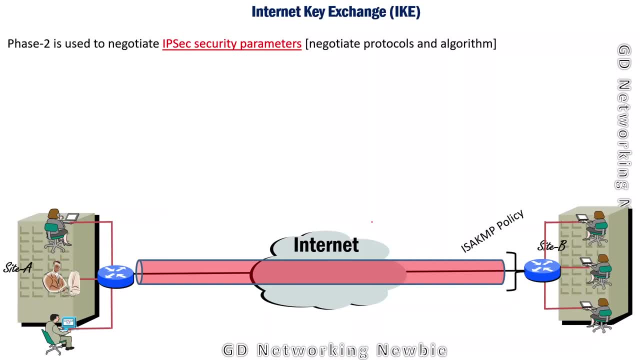 negotiate IP security parameters. So now we have this tunnel from phase one, We already have this tunnel And now this tunnel is actually is defined. It has defined the IP security parameters, some ICChem policy- we can call them ICChem policy- and once this tunnel is there, now in phase two, 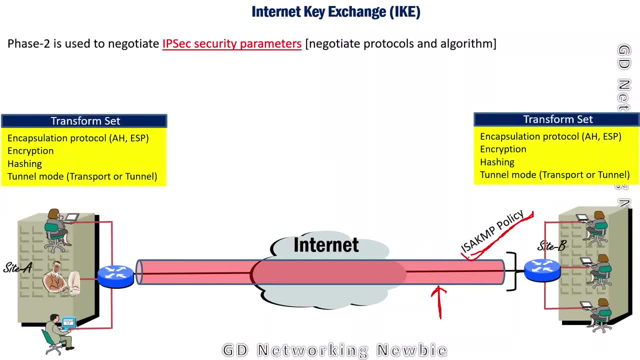 they negotiate IP security parameters. so in those IP security parameters they can, for example, decide about the encapsulation protocol, like AH or ESP- and we'll discuss about AH and ESP in our next video, otherwise video will be long- and then they also discuss and decide about encryption as well. 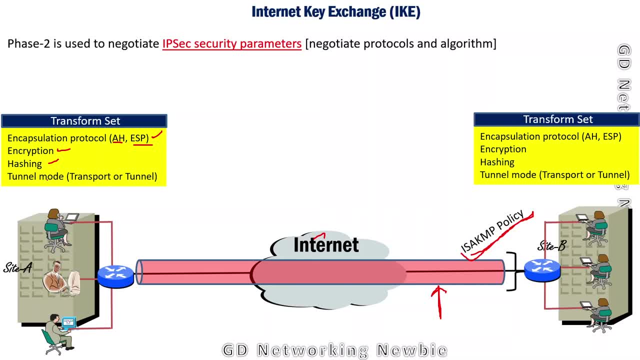 as hashing and the tunnel mode, whether they want to use transport mode or the tunnel mode, and so both of the nodes they need to agree or they need to negotiate these protocols as well as algorithm, and then, once they are done with that, we will have a common IPsec transform set. 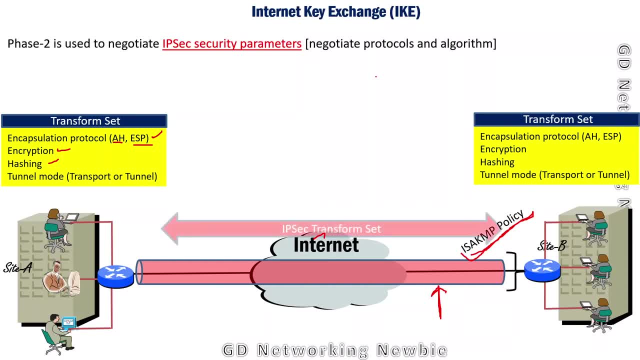 between these two points, between two these pairs, like in our case, between these two routers. now, within that, the tunnel which was created in first phase. in the second phase we have IPsec policy, which has been exchanged using the previous tunnel which was given in phase one. so 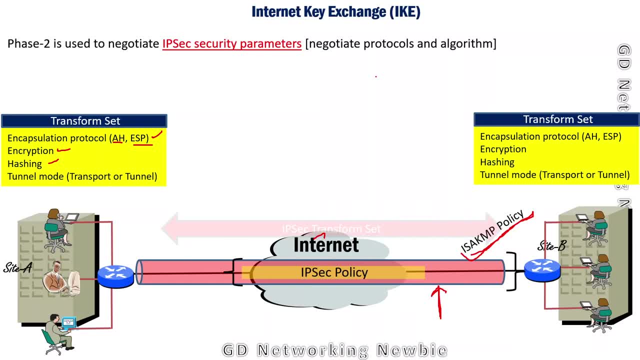 now we have this IPsec policy and now this IPsec policy will be used for our for, for sending our data securely. it means two phase. first phase was created to decide the IPsec policy and once the IPsec policy is there, once the IPsec policy is created, that IPsec policy will be used to securely. 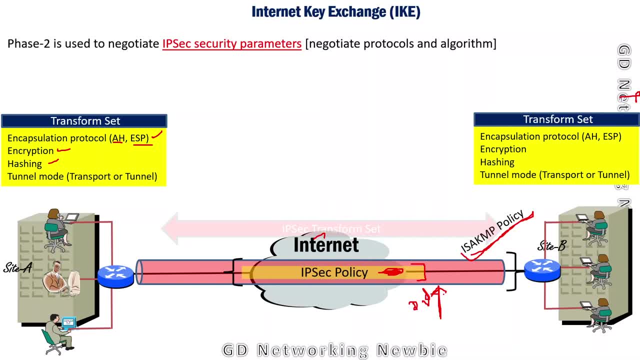 transmit our data. now we can exchange our data, and then this depends upon the lifetime of this connection, and then we can terminate these connections. so these were the two phases of ike, internet key exchange and those, these, uh, these two phases after these two phases, both of the end.